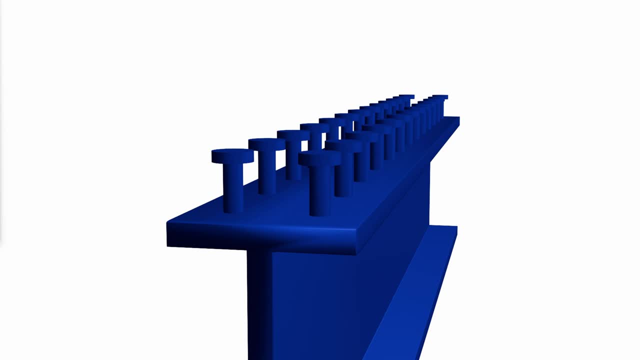 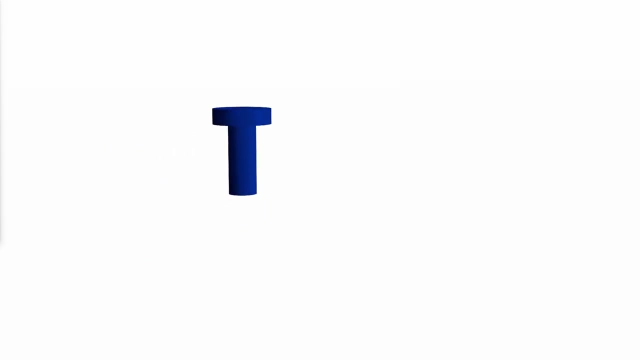 each location if the flange is wide enough to accommodate them, which depends on the allowable spacing. One reason for the popularity of steel-headed stud anchors is their ease of installation. It is essentially a one-worker job, made possible by an automatic tool that allows the operator to position the stud and weld it to the beam. 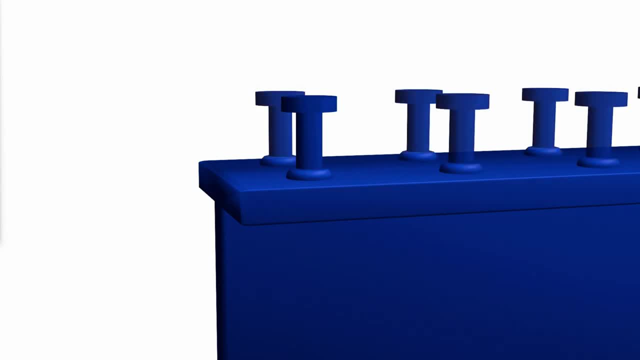 For example, in the case of a messed up beam, it can be used to make a new flange from the bottom of the comb. A number of anchors will be required to make a beam fully composite. Any fewer than this number will permit some slippage to occur between the steel and concrete Such a beam. 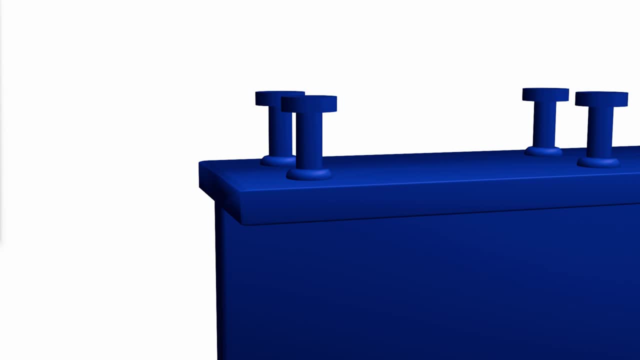 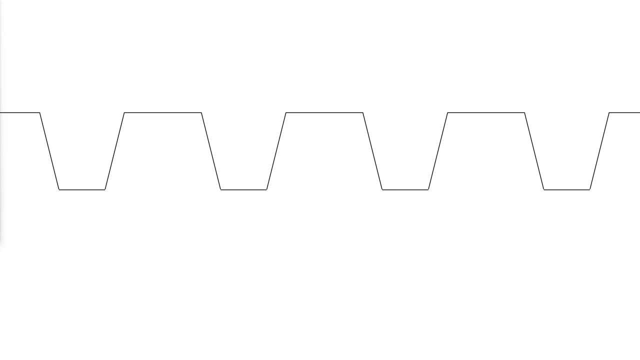 is said to be partially composite. In this video we will discuss only fully composite beams. Most composite construction in buildings utilizes formed steel deck which serves as a formwork for the beam. It is also made available in the agricultural market work for the concrete slab and is left in place after the concrete cures. 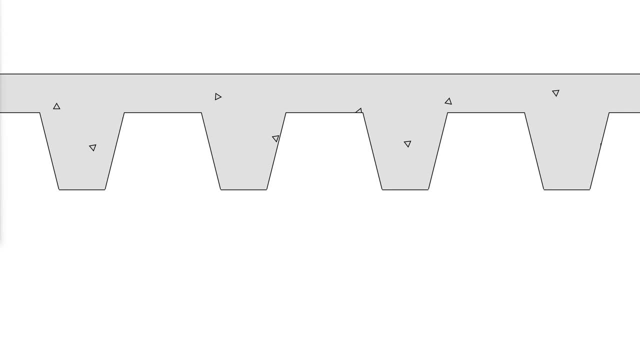 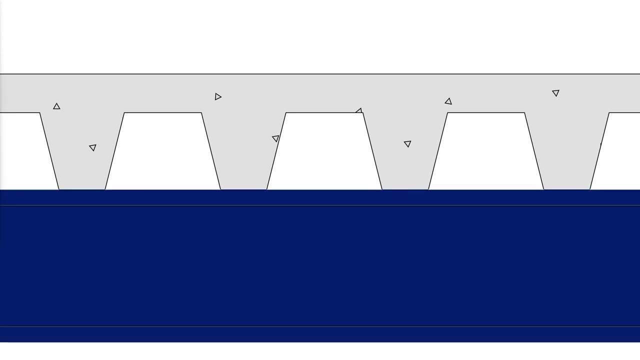 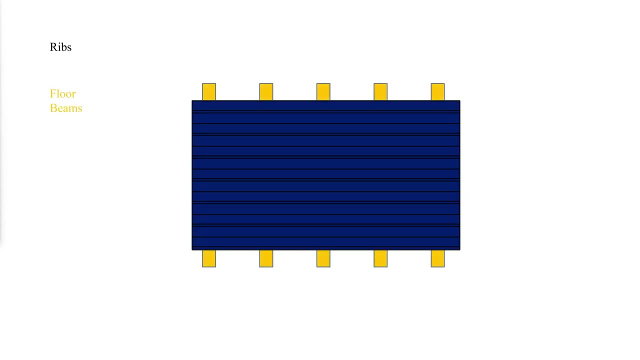 This metal deck also contributes to the strength of the slab. The deck can be used with its ribs oriented either parallel or perpendicular to the beams. In the usual floor system, the ribs will be perpendicular to the floor beams and parallel to the supporting girders. 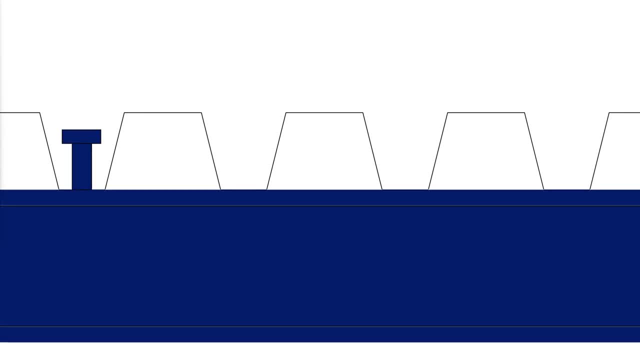 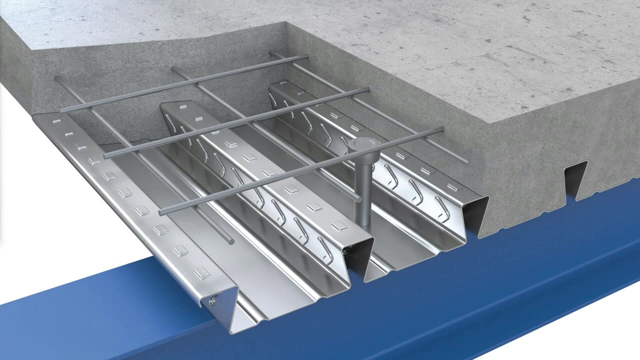 The studs are welded to the beams from above through the deck. Since the studs can be placed only in the ribs, their spacing along the length of the beam is limited to multiples of the rib spacing. Almost all highway bridges that use steel beams are of composite construction and composite. 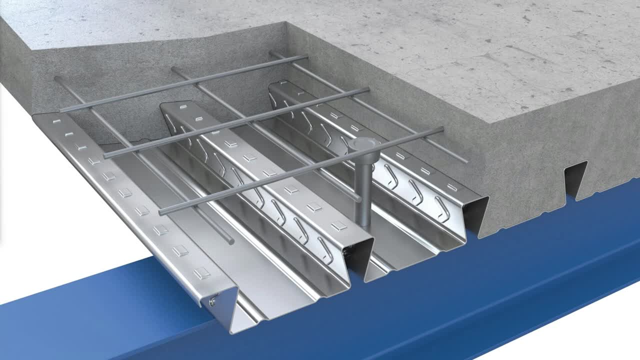 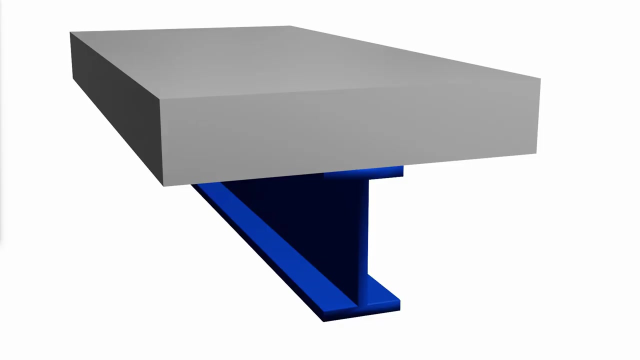 beams are frequently the most economical alternative in buildings. Although smaller, lighter rolled steel beams can be used with composite construction, this advantage will sometimes be offset by the additional cost of the studs. Even so, other advantages may make composite construction attractive: Shallower beams can be used and deflections will be smaller than with conventional non-composite. 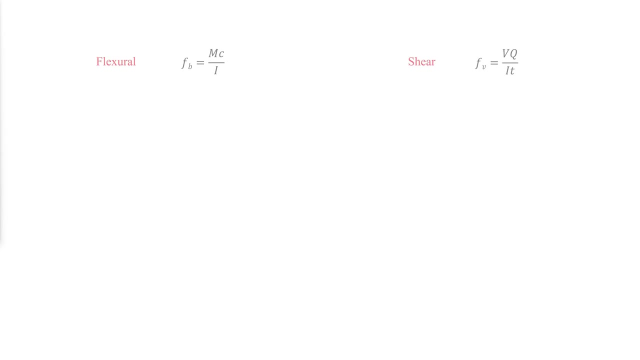 construction, Flexural and shearing stresses in beams of homogeneous materials can be computed from the following formulas: A composite beam is not homogeneous, however, and these formulas are not valid To be able to use them. we can theoretically convert the concrete into an amount of steel. 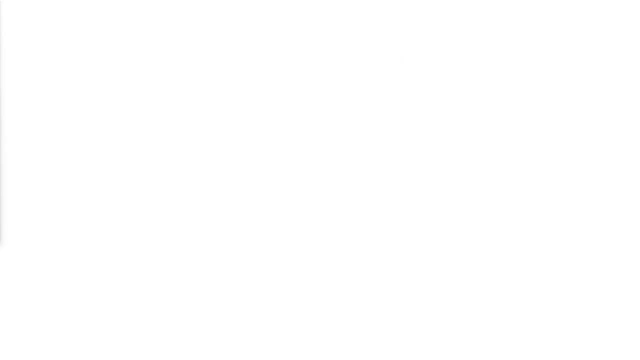 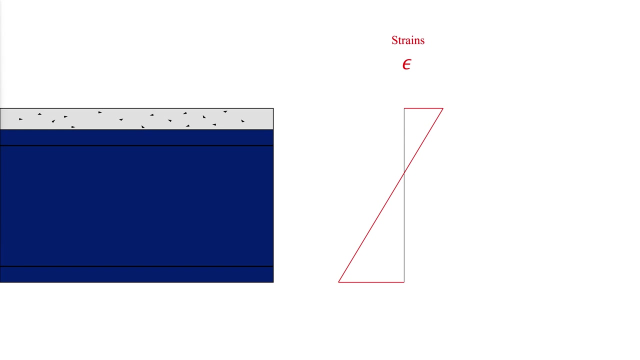 that has the same effect as the concrete. This procedure requires the strains in the fake steel to be the same as those in the concrete it replaces. If the slab is properly attached to the rolled steel shape, the strains will be as shown with cross sections that are plain before bending, remaining plain after bending. 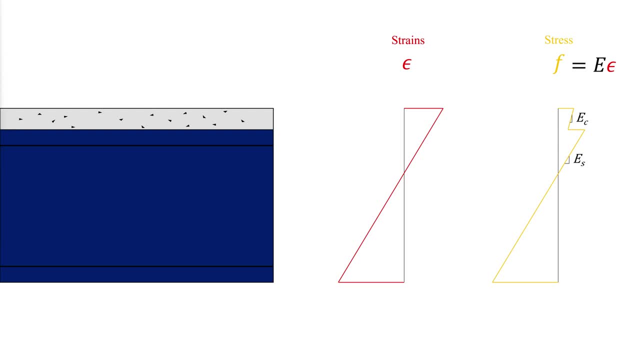 However, because the modulus of elasticity of concrete differs from that of steel, the stress distribution will not be linear and continuous, with a jump happening at the interface between steel and concrete. We first require that the strain in the concrete at any point be equal to the strain in any 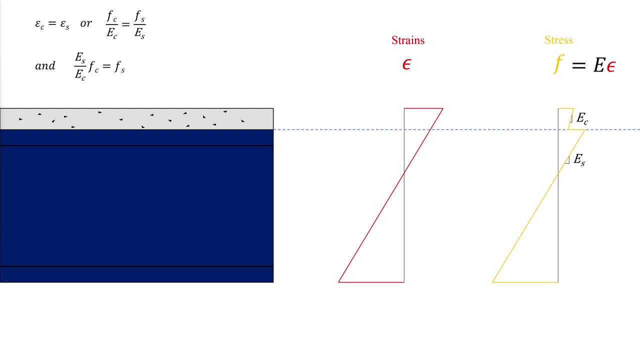 replacement steel. at that point, AISC I2.1b gives the modulus of elasticity of concrete as the unit weight of concrete to the power of 1.5 multiplied by the square root of the 28-day compressive strength of the concrete. 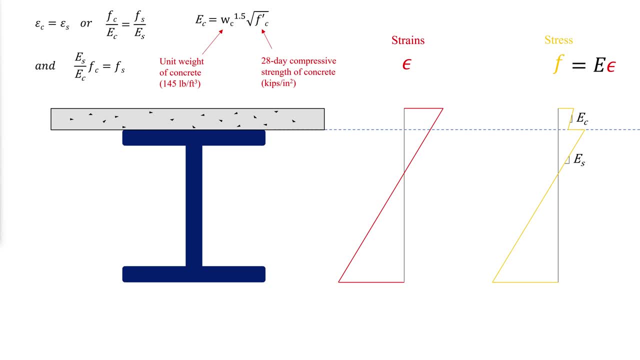 To determine the area of steel that will resist the same force as the concrete, divide the concrete area by the ratio of elastic modulus of steel to that of the concrete, called N. To transform the concrete area A sub C, we must divide by N, The most convenient way. 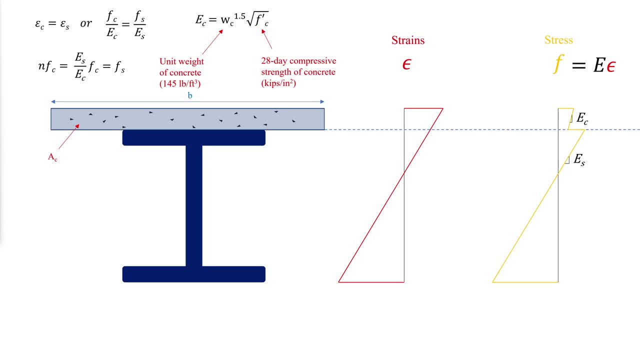 to do this is to divide the width by N and leave the thickness unchanged. Doing so results in the homogeneous steel section shown. To compute stresses. we locate the neutral axis of this composite shape and compute the corresponding moment of inertia. We can then compute bending stresses with the flexure force. 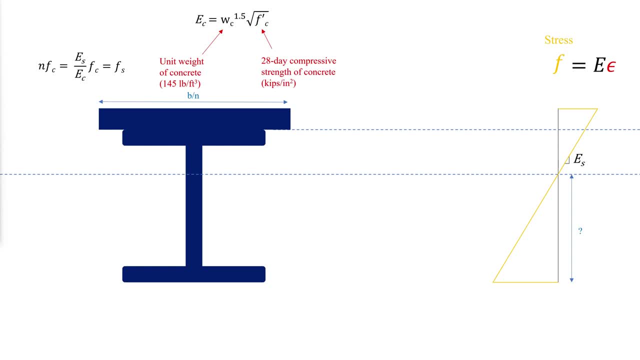 We can then compute bending stresses with the flexure force. We can then compute bending stresses with the flexure force. How do we solve the stress? первon اور blight. Thank you so much. And let's review the flexure formula, where m is the applied bending moment and I sub T.